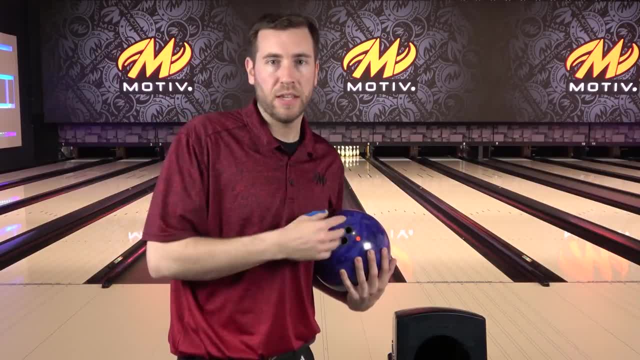 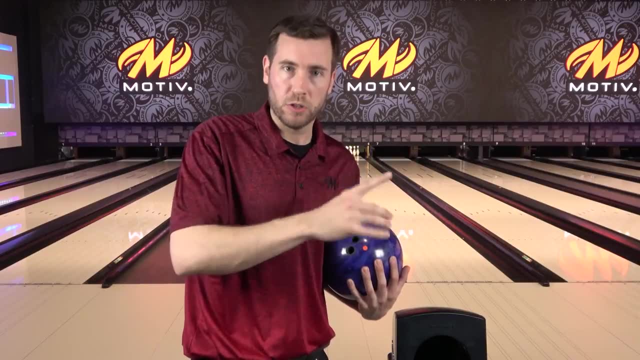 just to figure out what the what the pattern kind of feels like. If it feels really long, if my ball never hooks, or if I see where the friction starts, that means you know, I know where I need to get my ball to down the lane. So, like I said, I'm gonna start first arrow, see what it does. 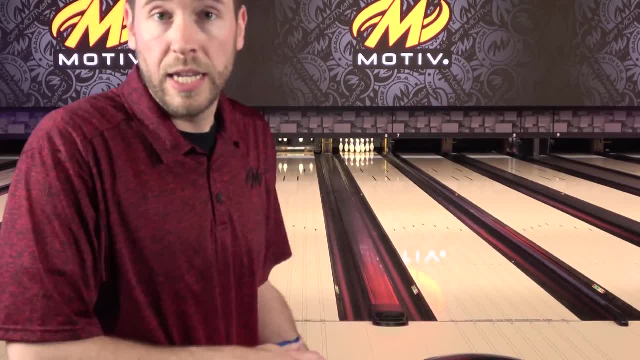 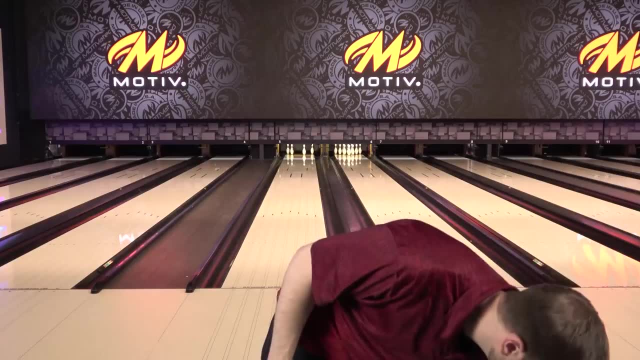 Okay. so the ball went pretty far down the lane before it hooked, but it did hook quite a bit down the lane. So now I'm gonna go to second arrow, you know up ten, Kind of see what that gives me. but that tells me right away that my ball is. 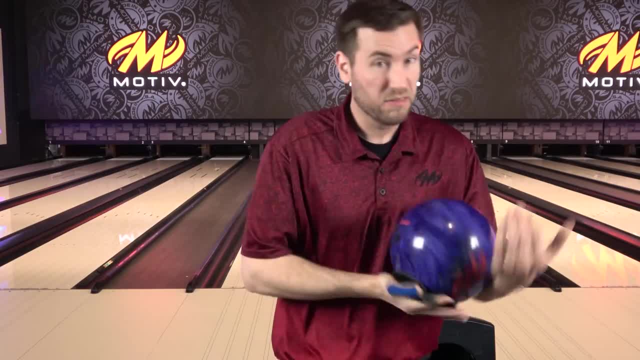 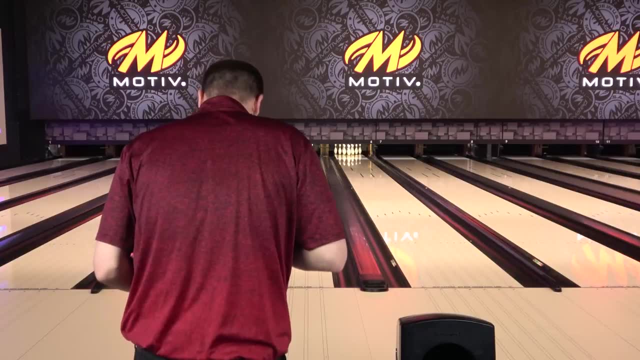 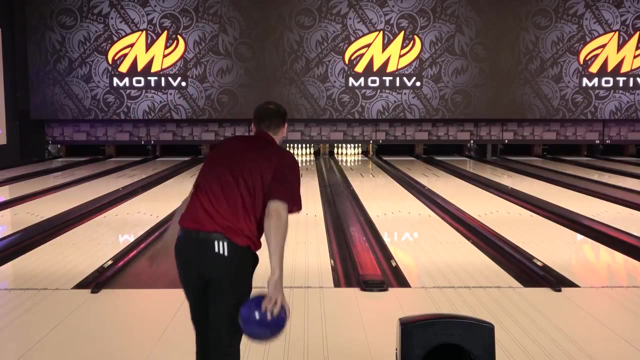 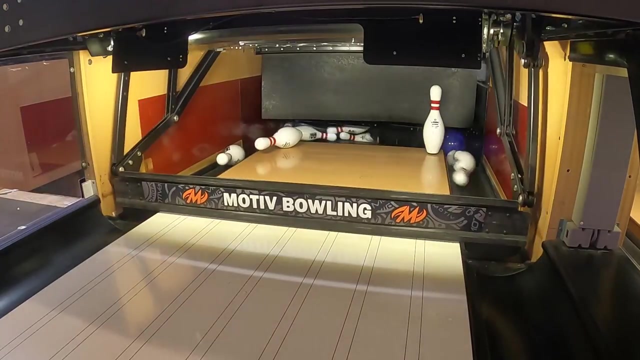 storing quite a bit energy and using it all down lane, So I feel like there's quite a bit of oil out here, So I wouldn't be surprised if this next ball doesn't hook. So second arrow: Okay, so that was pretty close. actually. I hit the pocket and the messenger in. 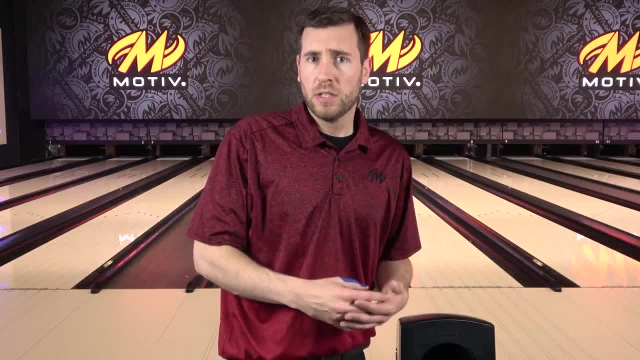 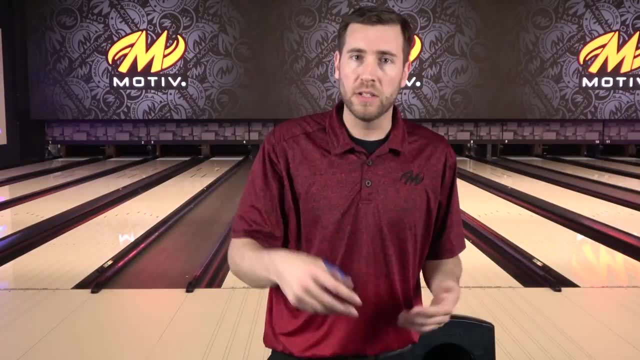 front of the ten. It just means my ball is a little bit behind the head pin, So that's a good sign. when I see something like that, when I have no idea what the pattern is doing, It just tells me the ball is a little bit too far down the lane. when it 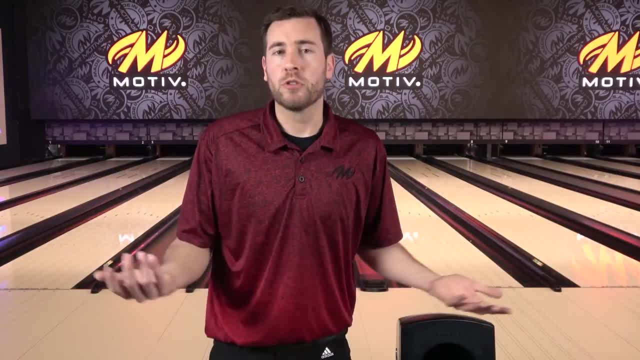 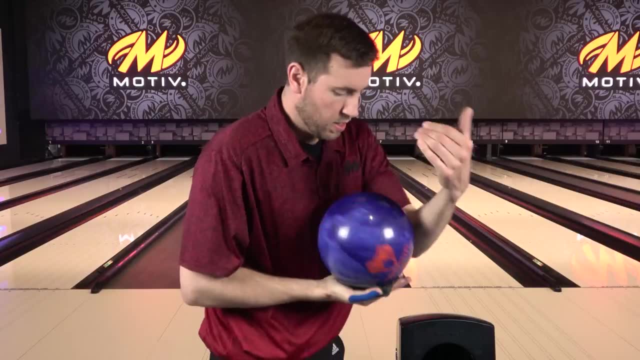 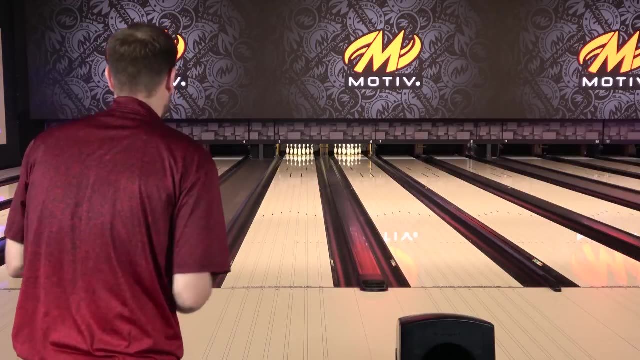 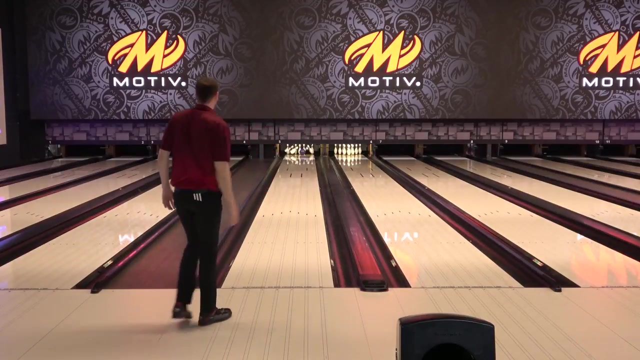 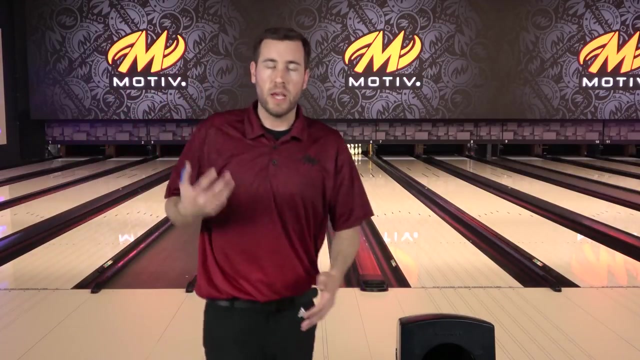 tries to change directions. So from there I might actually throw a stronger ball in that same zone, But I am gonna try 15.. So we're gonna go to third arrow. Let's see what this does for me. All right, so there saw me wrap ten Ball skidded, you know, skidded down lane pretty. 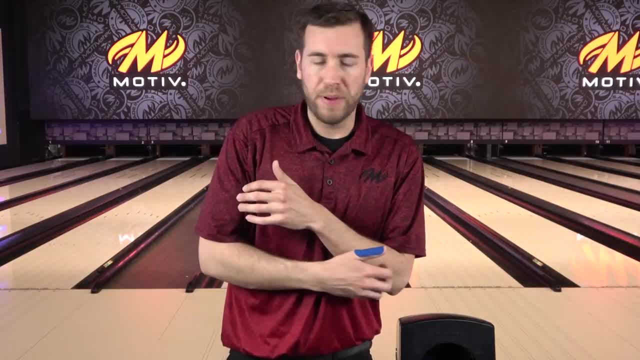 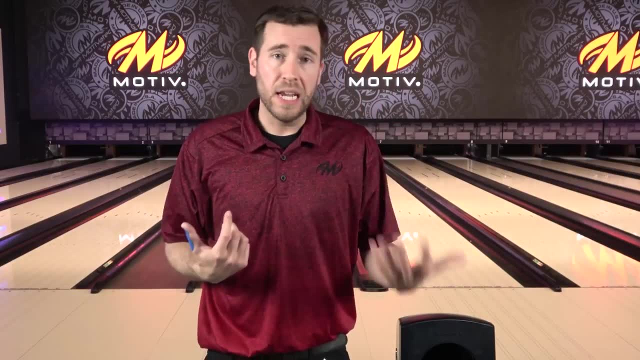 easy, Had no problem. So it definitely feels like it's a longer pattern to me That one just was in two much oil and couldn't change directions hard enough to get the ten out. So from there I would probably go back to the right where I was close, you know, up ten.